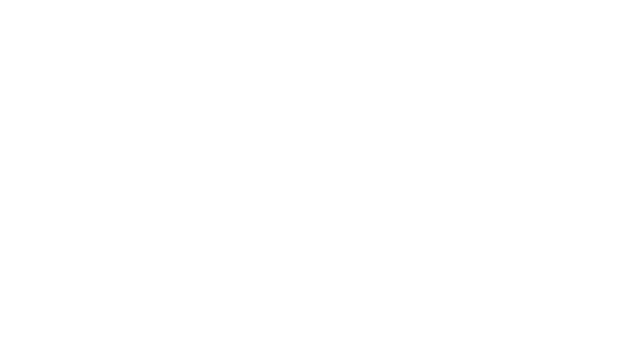 In this video we're going to take a look at metallic bonding, which is the type of bonding you get between metal atoms, and we'll see how this gives rise to the characteristic properties of metals. Then, lastly, we'll consider how alloys differ from pure metals. 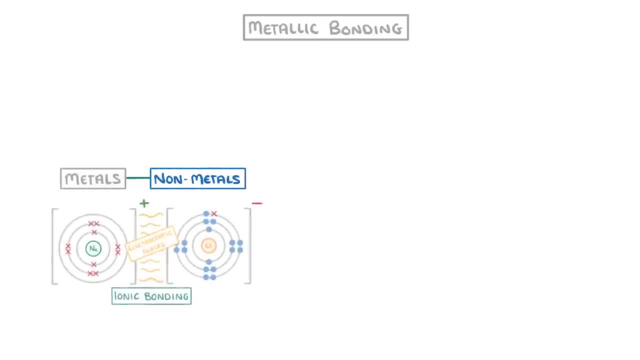 To recap, we've already seen that metals bond to non-metals through ionic bonding and that non-metals bond to other non-metals through covalent bonding. Now we turn to how metals bond to other metals, which we call metallic bonding. 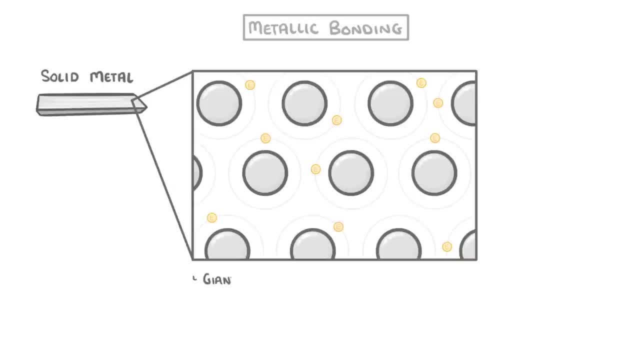 If we think of a solid metal, it basically consists of a giant structure of atoms that are arranged in a regular pattern. In this picture, we've shown each atom surrounded by the electrons in its outermost shell. When all these atoms are together in a metal, though, 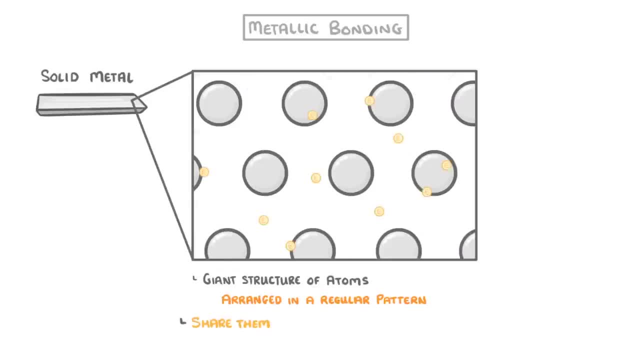 they actually give up these outer shell electrons. This means that the atoms will all become positive ions because they've lost negative electrons And because those electrons are now free to move about, we call them delocalised electrons. So there will now be loads of strong electrostatic attraction between the positive ions and the 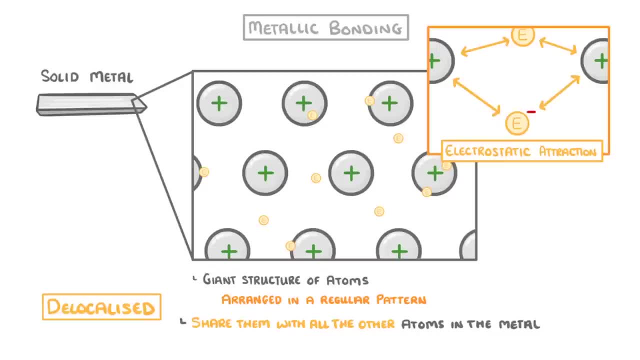 negative electrons, And it's these forces of attraction which hold everything together in a regular pattern, So we call this metallic bonding. This gives the overall metal strength and means that most metallic structures have high melting and boiling points, so are solid at room temperature. 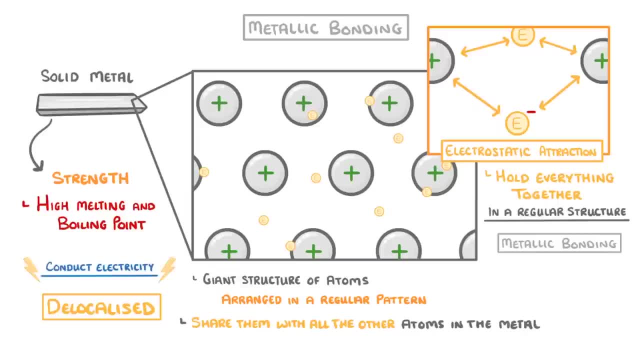 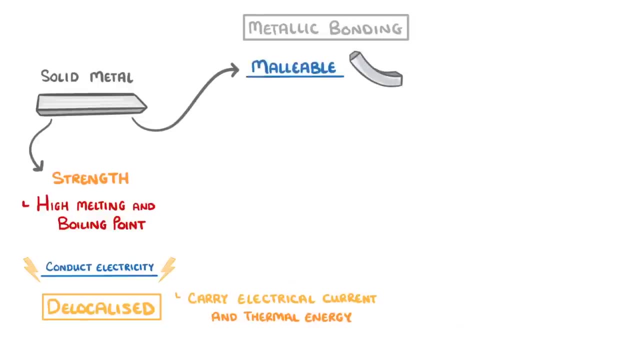 They are also good conductors of electricity and heat, because the delocalised electrons can carry electrical current and thermal energy throughout the structure. Another important property is that metals are malleable. Metals are malleable, which means that they can easily be bent or hammered into shapes. 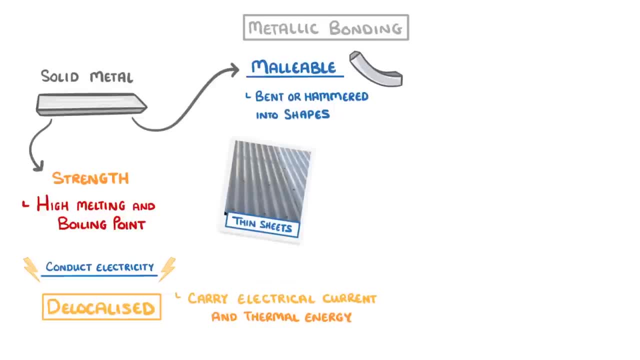 for example, into thin sheets. This can be a bit confusing, because we think of metals as being strong, and in many ways they are. But the fact that metals have such a regular structure means that the different layers can slide over one another, so they're not.